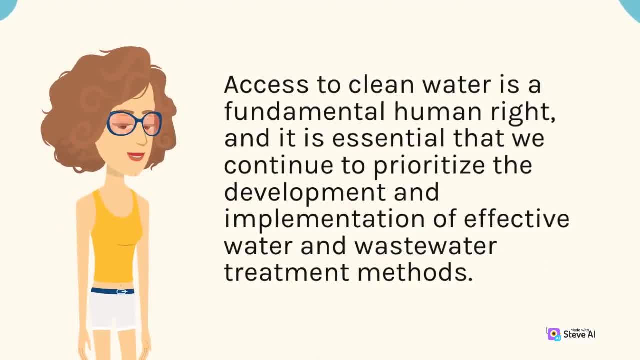 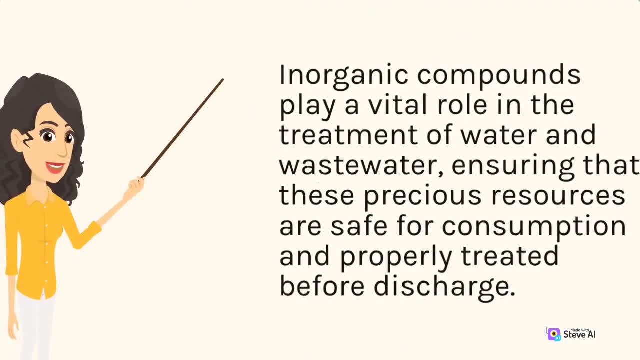 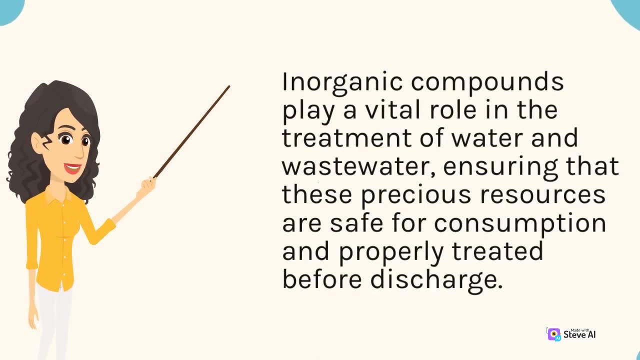 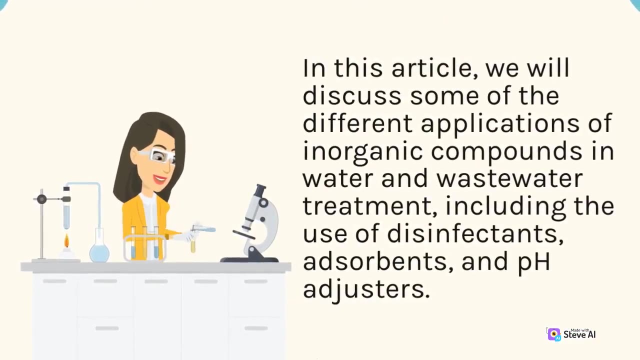 Inorganic compounds play a vital role in the treatment of water and wastewater, ensuring that these precious resources are safe for consumption and properly treated before discharge. In this article, we will discuss some of the different applications of inorganic compounds in water and wastewater treatment, including the use of disinfectants, adsorbents and pH adjusters. 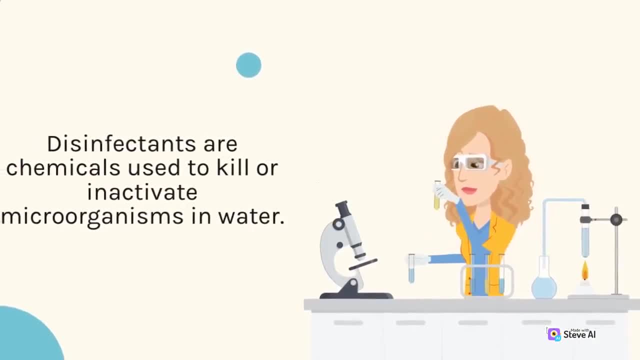 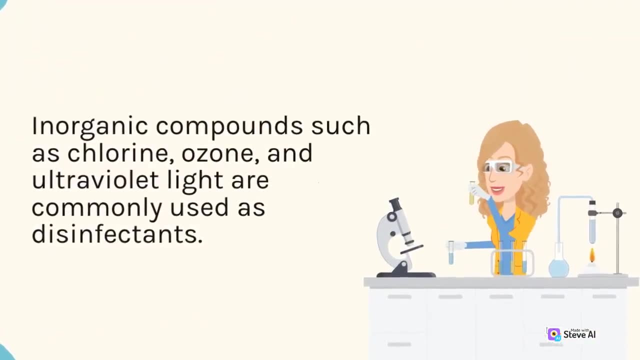 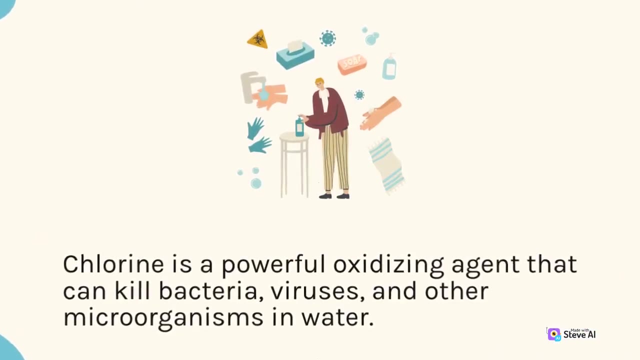 Disinfectants are chemicals used to kill or inactivate microorganisms in water. Inorganic compounds such as chlorine, ozone and ultraviolet light are commonly used as disinfectants. Chlorine is a powerful oxidizing agent that can kill bacteria, viruses and other microorganisms in water. 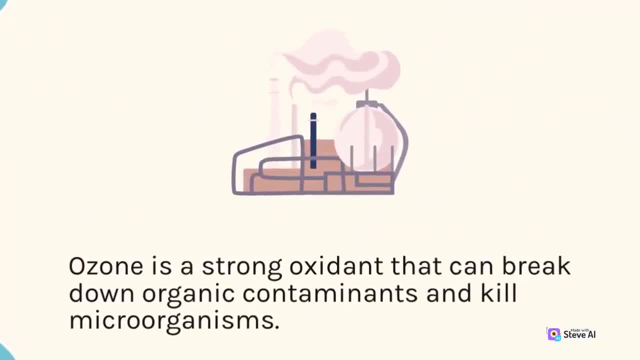 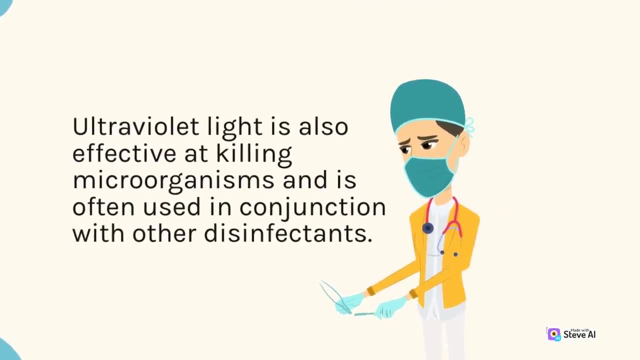 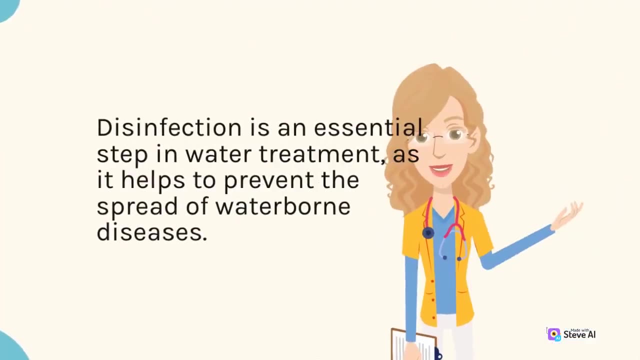 Ozone is a strong oxidant that can break down organic contaminants and kill microorganisms. Ultraviolet light is also effective at killing microorganisms and is often used in conjunction with other disinfectants. Disinfection is an essential step in water treatment, as it helps to prevent the spread of waterborne diseases. 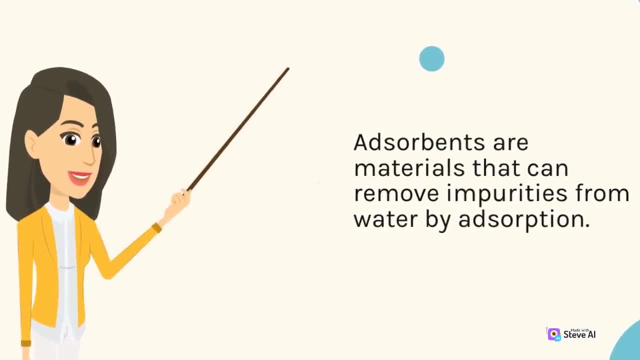 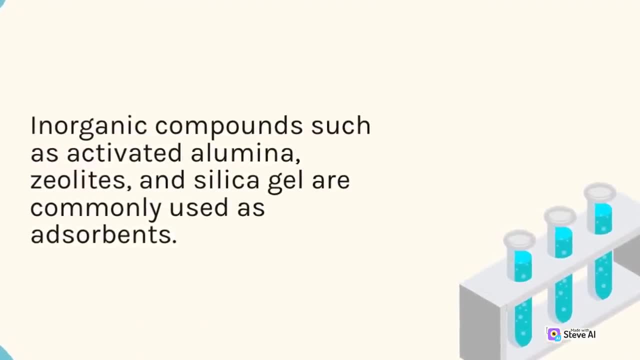 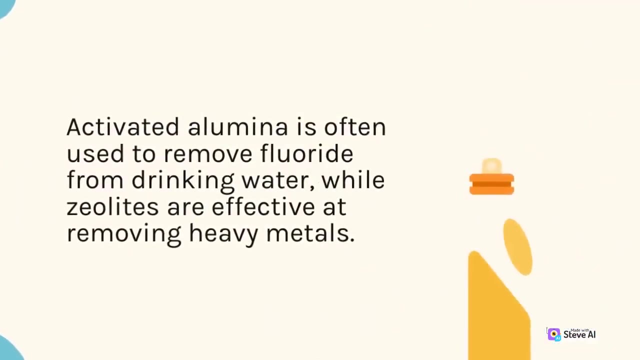 Adsorbents are materials that can remove impurities from water by adsorption. Inorganic compounds such as activated alumina, zeolites and silica gel are commonly used. Activated alumina is often used to remove fluoride from drinking water, while zeolites are effective at removing heavy metals. 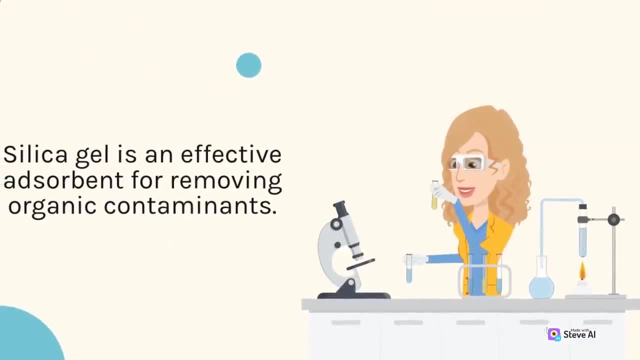 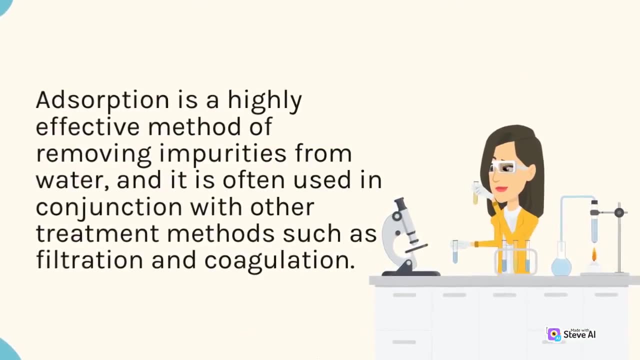 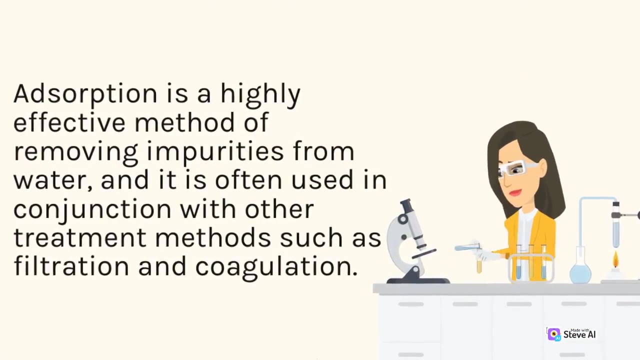 Silica gel is an effective adsorbent for removing organic contaminants. Adsorption is a highly effective method of removing impurities from water, and it is often used in conjunction with other treatment methods such as filtration and coagulation. pH adjusters are chemicals used to adjust the pH of water. 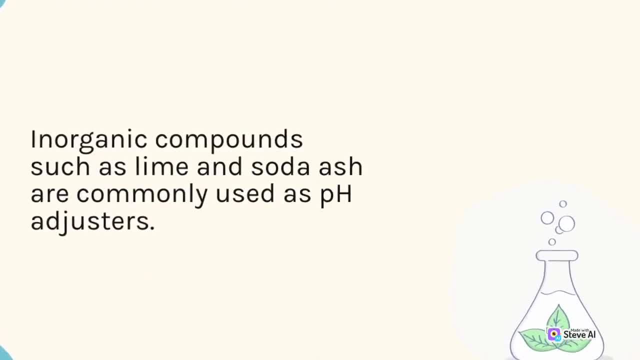 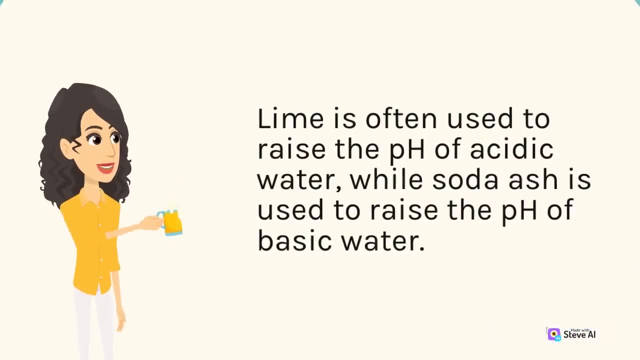 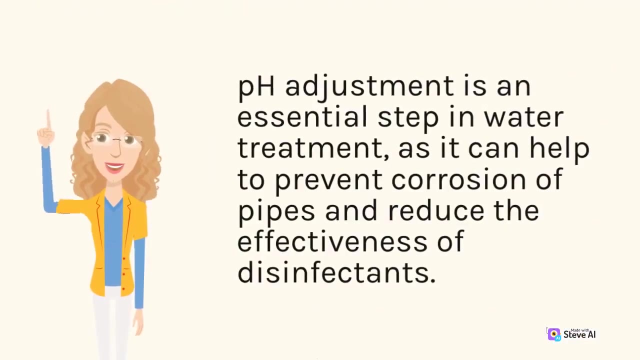 Inorganic compounds such as lime and soda ash are commonly used as pH adjusters. Lime is often used to raise the pH of acidic water, while soda ash is used to raise the pH of basic water. pH adjustment is an essential step in water treatment, as it can help to prevent corrosion of pipes and reduce the effectiveness of disinfectants.